23., 24., 25., 26., 27., 28., 29., 30., 31., 32., 33., 33., 34., 34., 35., 36., 36.. 37., 38., 39., 39., 40., 41., 42., 43., 43., 44., 44., 45., 46., 46., 47., 48., 49.. 50., 51., 52., 52., 53., 54., 55., 56., 57., 58., 59., 60., 61., 62., 63., 62., 63.. 64., 65., 66., 67., 68., 67., 68., 69., 67., 68., 69., 69., 70., 71., 72., 73., 74.. 75., 76., 75., 76., 77., 78., 78., 79., 79., 80., 80., 81., 82., 82., 83., 83., 84.. 84., 85., 86., 87., 86., 87., 88., 88., 89., 90., 92., 92., 93., 95., 92., 94., 93.. 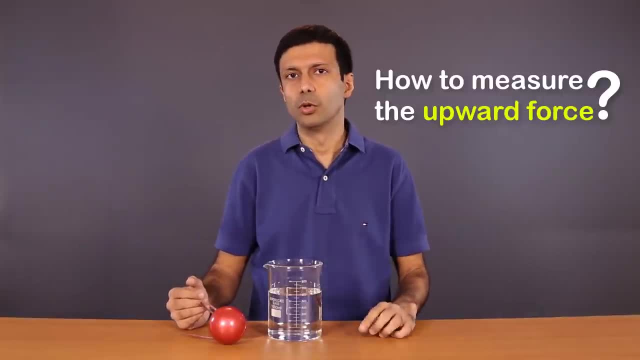 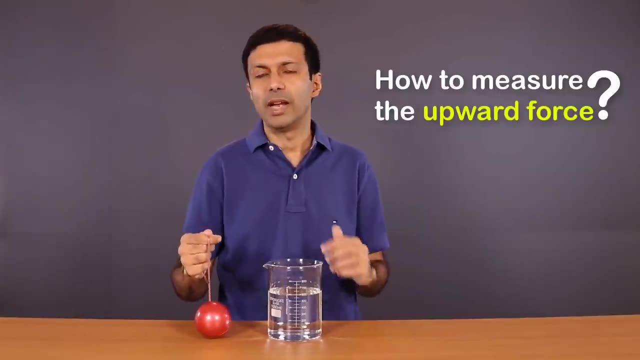 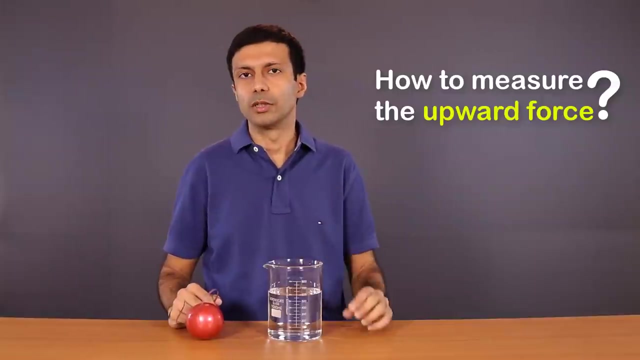 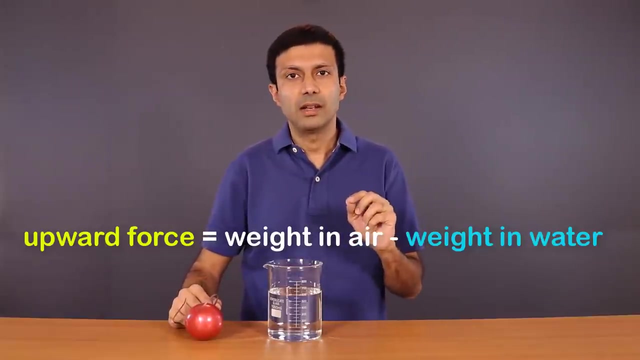 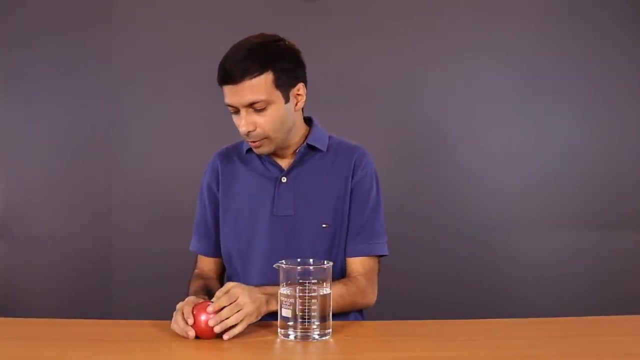 93., 95., 95., 96., 97. 0.. of upward force. Let's go ahead and try it out. For this experiment, I've taken this hollow ball and I've filled it with coins here to make it heavy. Let's. 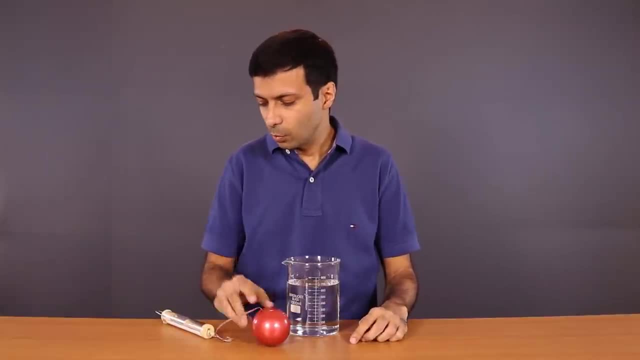 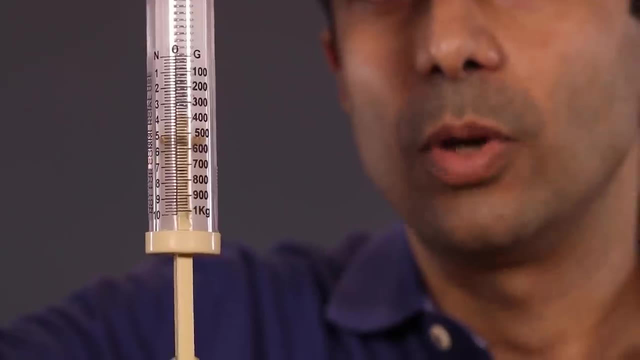 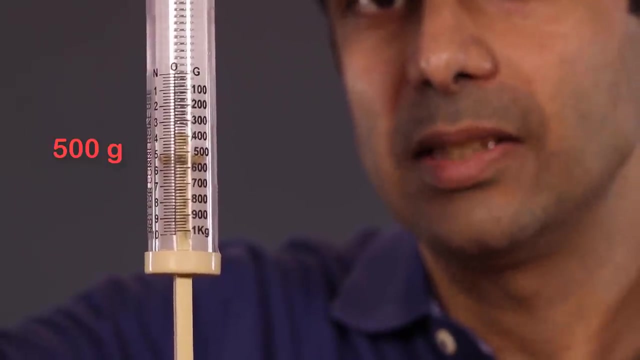 measure the weight of this ball which is filled with coins, with the help of this spring balance. So let's see what is the weight here. So, as you can see, here the weight is 500 grams. or, to be more precise, in physics the weight is 500. 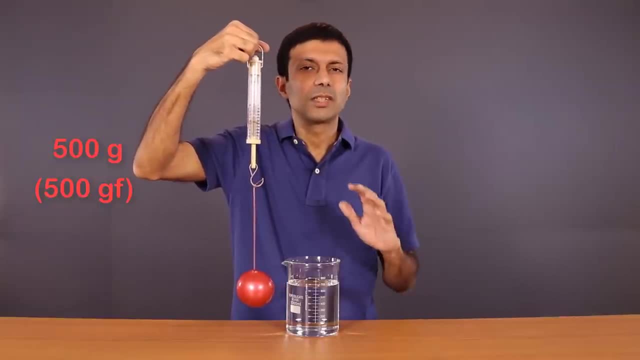 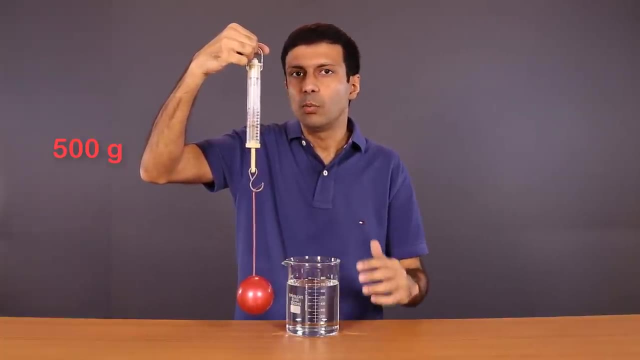 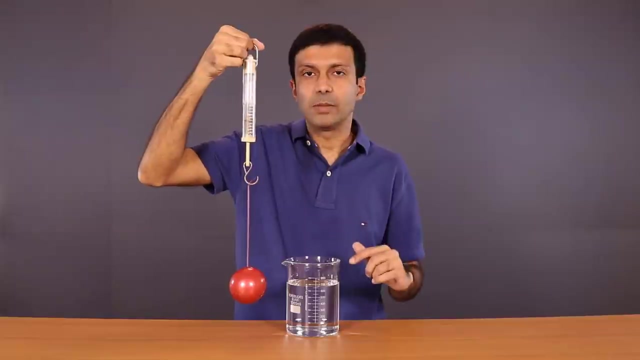 gram force, But for this video we'll just keep things simple and use gram as the unit of weight, And this weight is known as the real weight of the ball because it is the weight in air. Now I'm going to immerse this ball into this beaker of. 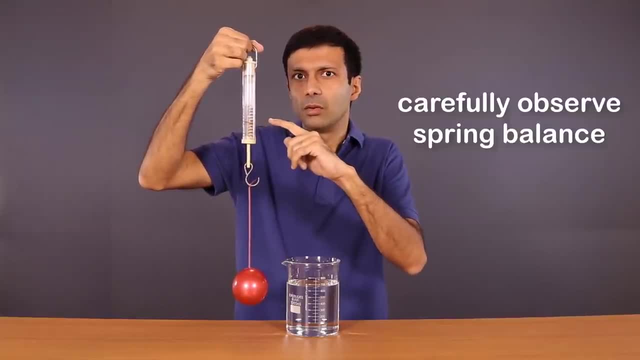 water and you carefully observe what is the reading of the spring balance. Now I'm going to immerse this ball into this beaker of water and you carefully observe what is the reading of the spring balance. Now I'm going to immerse this ball into this beaker of water and you carefully observe what is the reading of the spring balance. 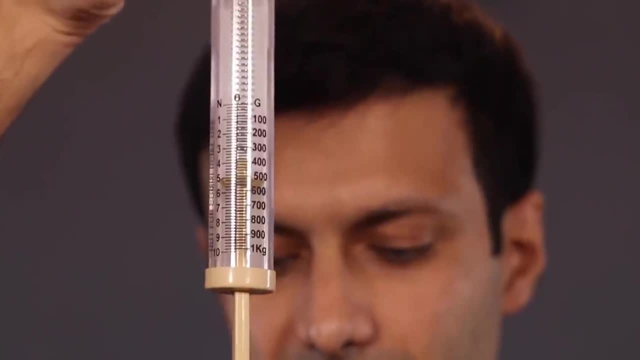 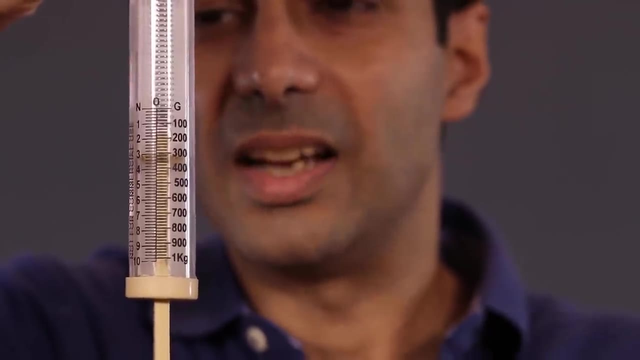 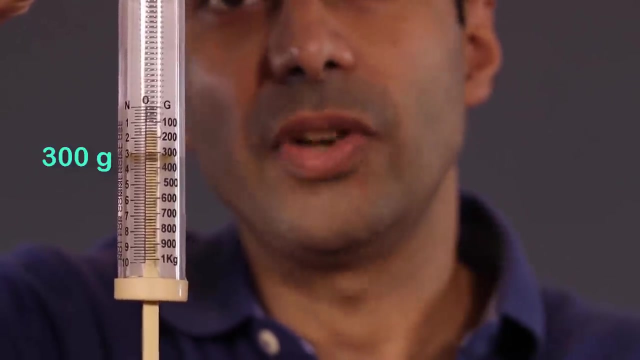 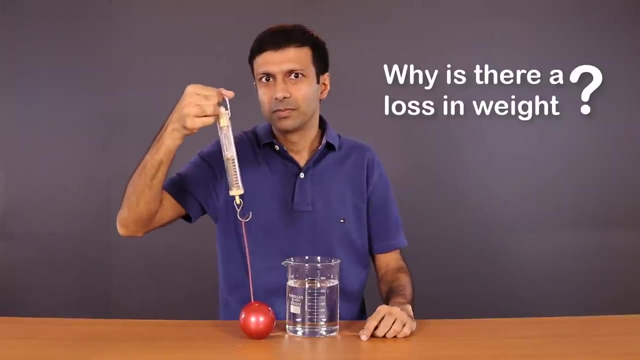 So I'm going to lower the ball here. So what did you observe? As you can see, the spring balance shows that the weight of the ball when it's immersed in water is now 300 grams. So there is a loss in weight when the ball is held in water. So why is that? It's because of the 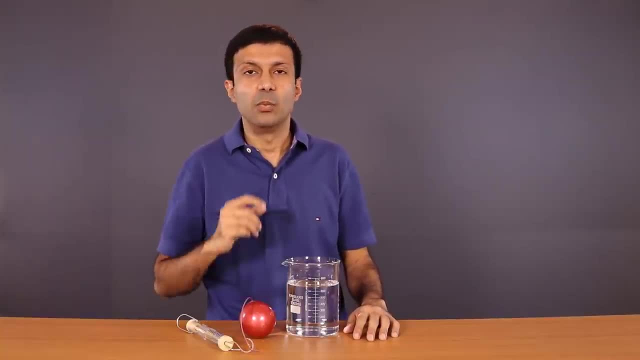 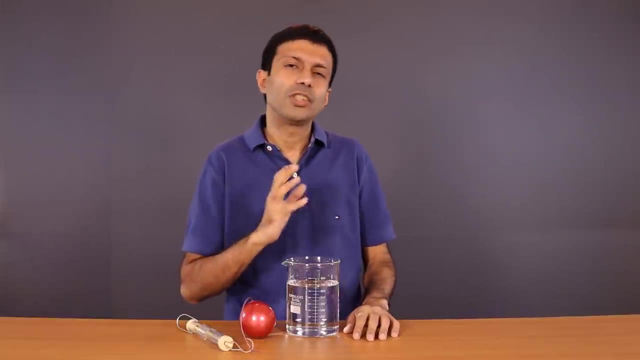 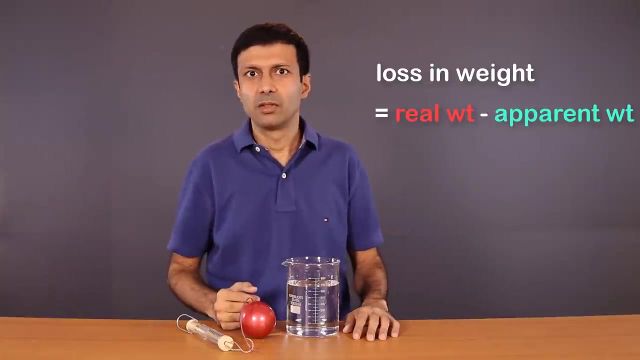 upward force of the water. And the weight in water is called as the apparent weight because the ball seems to lose weight. And how much is this apparent loss in weight? It's the real weight minus the apparent weight, So it's going to be 500 grams. 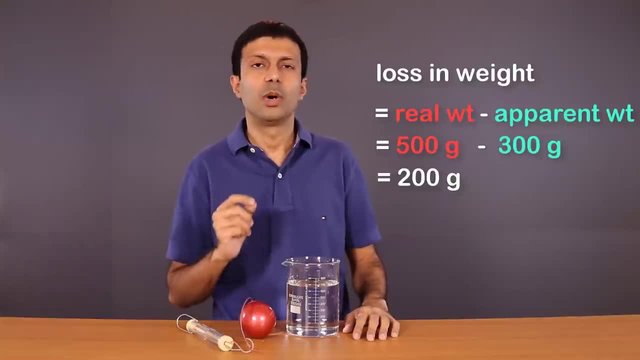 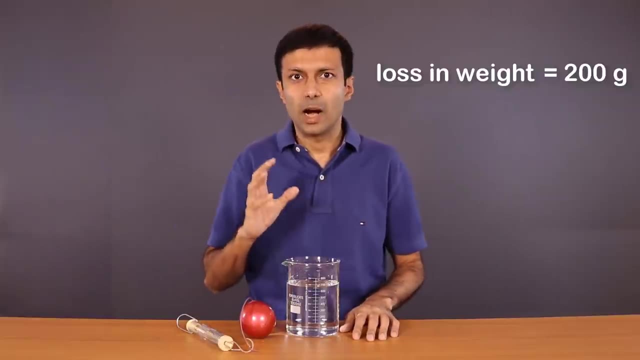 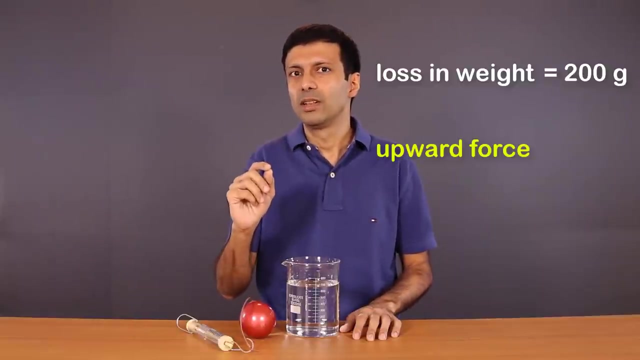 minus 300 grams, that's 200 grams. So the loss in weight is 200 grams and we note that the upward force is contributing to this loss in weight. So the upward force is actually the loss in weight, which is 200 grams, or, to be more precise, 200 gram. 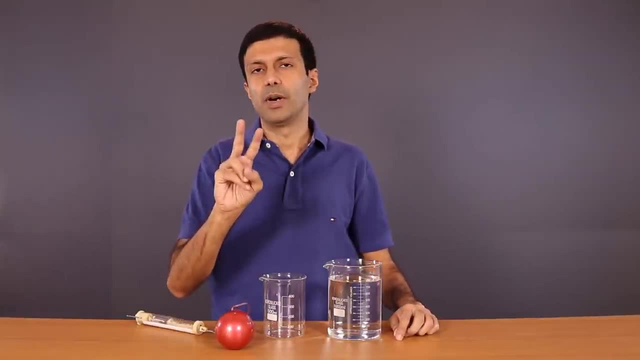 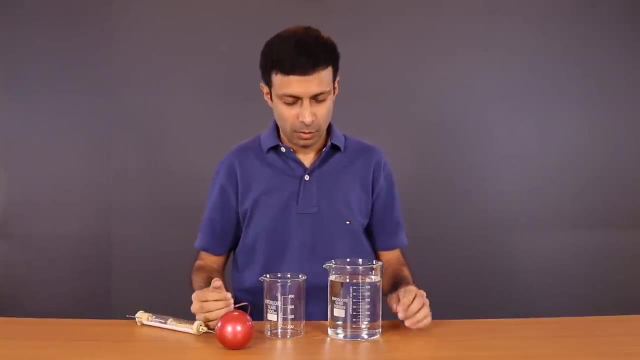 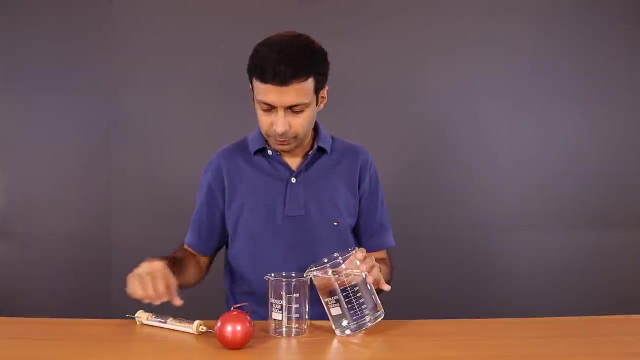 force. Now let's take a look at the second part, that the upward force is equal to the weight of the water displaced by it. So I'm going to go ahead and tilt this larger beaker so that the displaced water goes into the smaller beaker. So let's try it one more time. 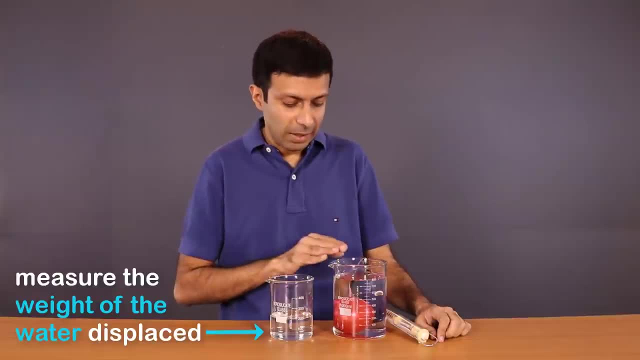 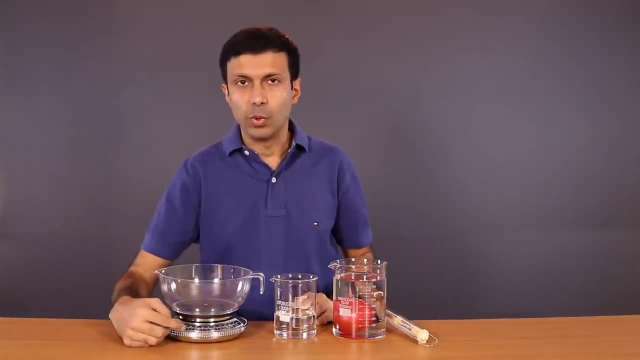 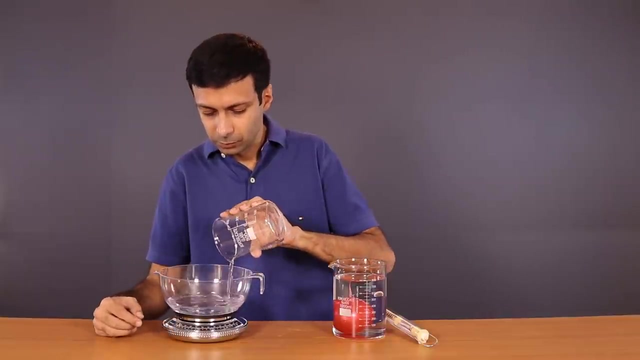 Let's measure the weight of the water displaced by it. So the upward force is equal to the weight of this water that has been displaced by this ball. So I'm going to pour this displaced water into the pan here with a weighing scale. So 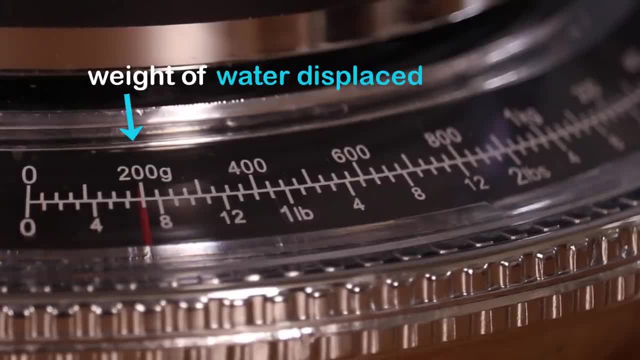 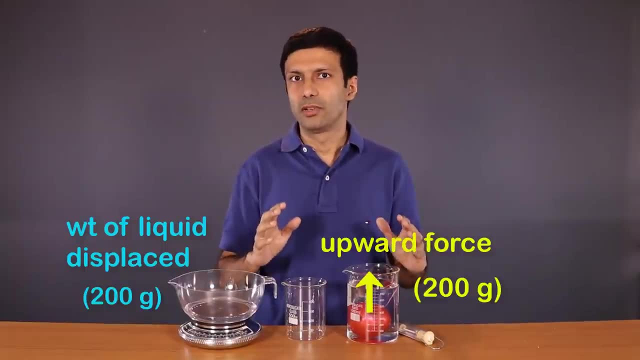 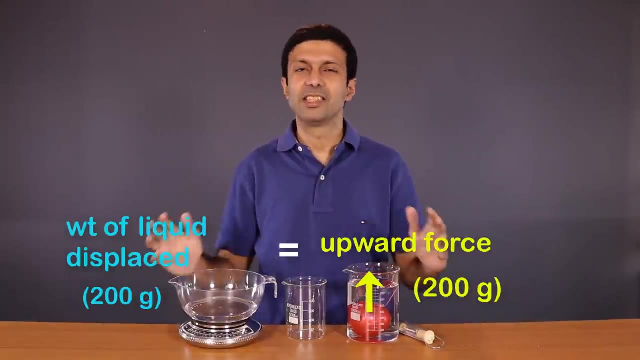 what is the weight of the water? As you can see, it's 200 grams. So the upward force and the weight of the liquid displaced are both 200 grams Or 200 gram force. So they are equal and Archimedes is correct. Now let's go back. 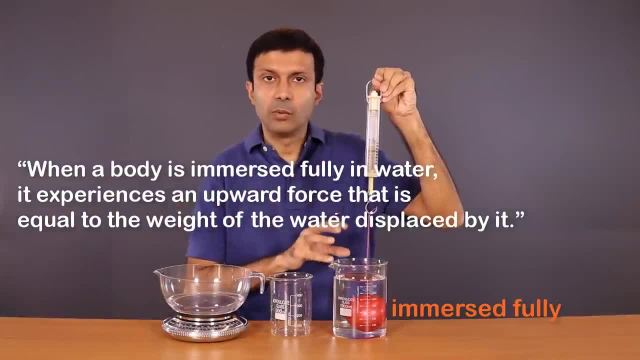 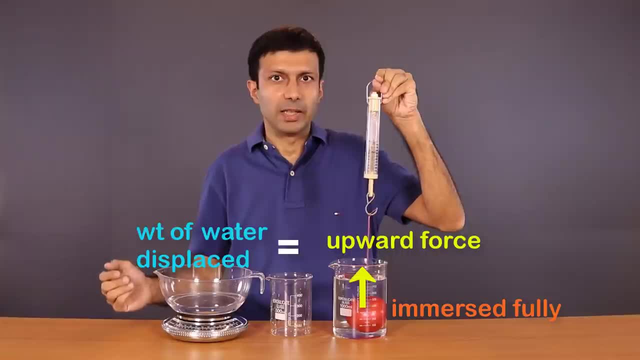 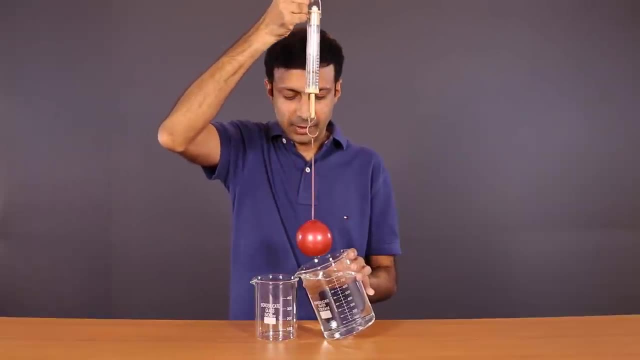 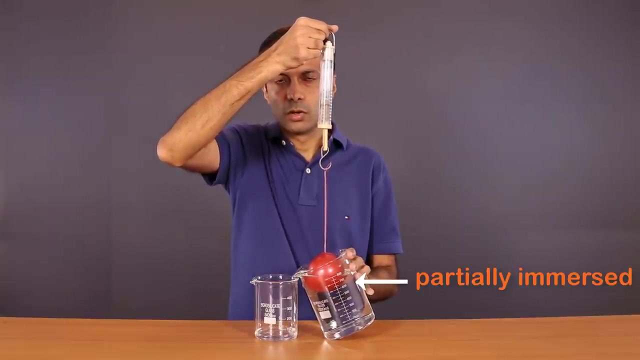 to our statement. When a body is immersed fully in water, it experiences an upward force that is equal to the weight of the water displaced by it. Archimedes principle also works for the partially immersed case. So for the case like this, where I have this ball partially immersed in water, So the upward force, which is 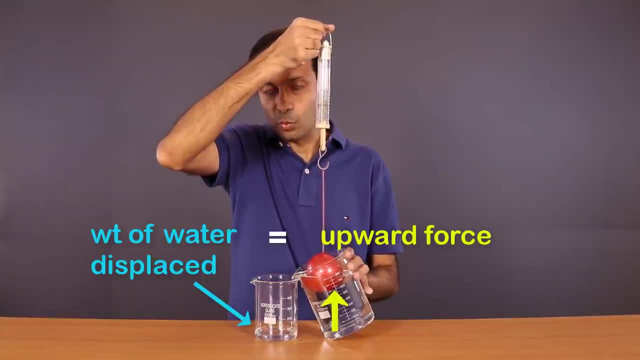 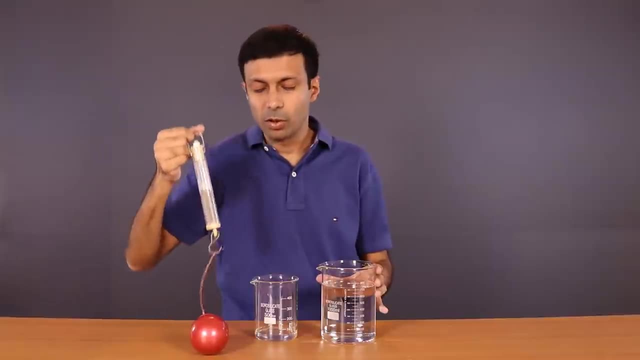 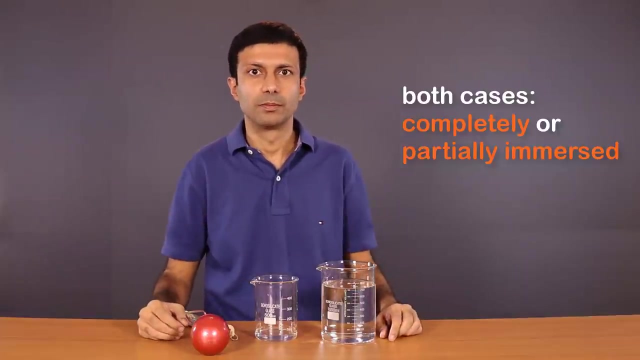 measured by the loss in weight here is equal to the weight of this water displaced. So Archimedes principle works for both the cases, whether the object is completely immersed in water or partially immersed in water, And in fact it works not only for water, but any. 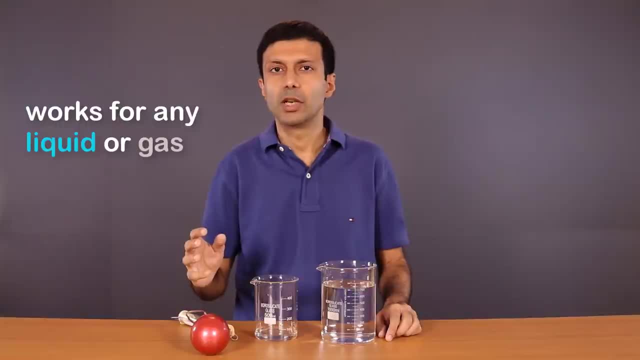 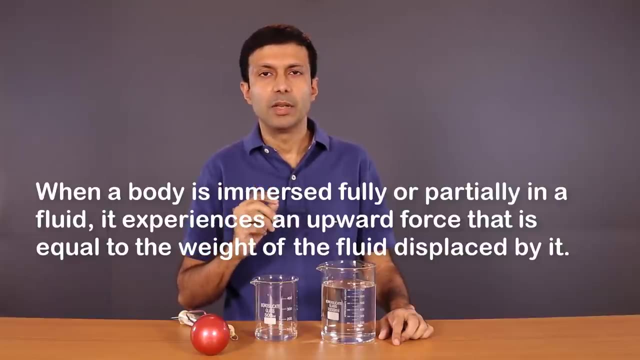 liquid and gas. So we can say that this principle works for any fluid. So the statement becomes: when a body is immersed fully or partially in a fluid, it experiences an upward force that is equal to the weight of the fluid displaced by it. So let's. 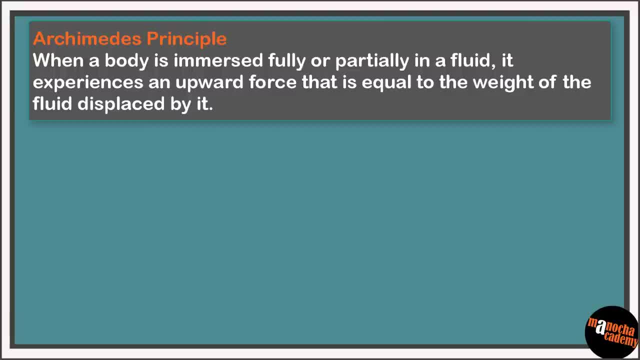 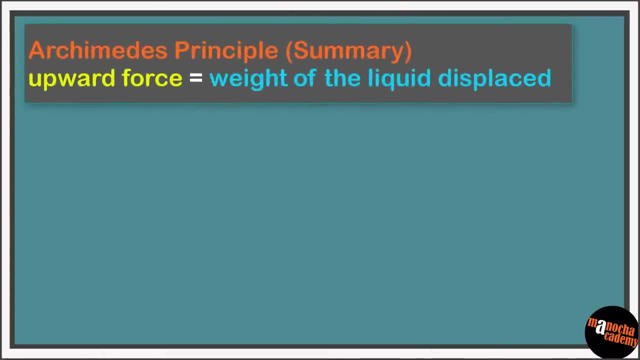 place Archimedes principle on our concept board. We can summarize his principle as: upward force is equal to the weight of the liquid displaced. We also saw in this video that the loss in weight of the body is equal to the real weight minus the apparent weight. 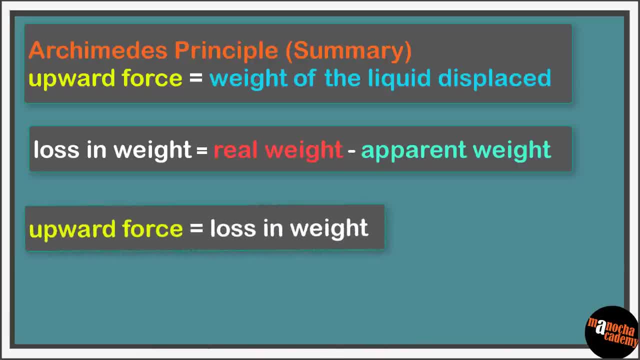 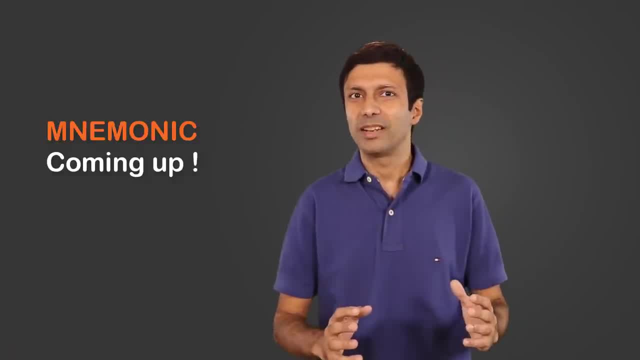 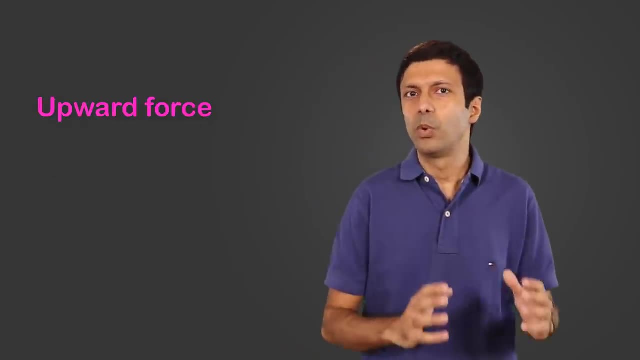 And this loss in weight was used to measure upward force, Since upward force and loss in weight are equal. Remember, I had promised a mnemonic at the beginning of this video to help you remember Archimedes principle. So, rather than upward force, you can remember. 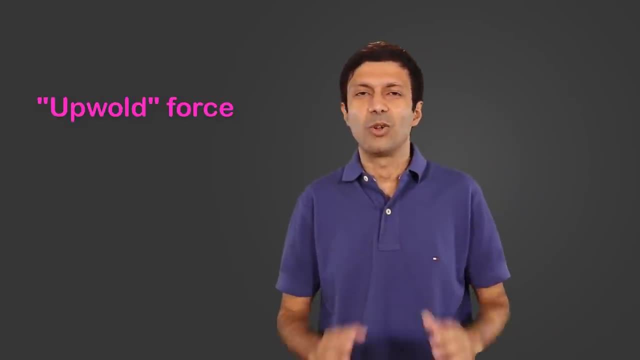 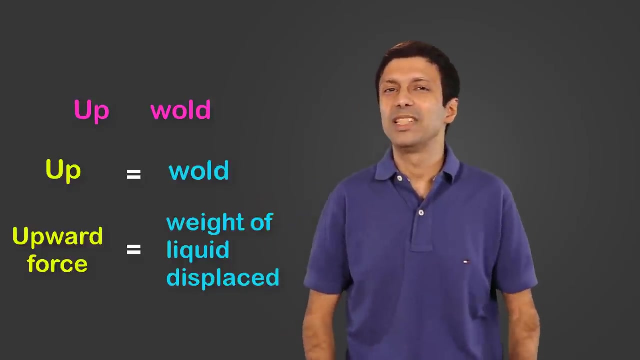 it as up-walled force. Now let's split the word. So we have up equal to walled. So that is: upward force is equal to the weight of the liquid displaced. I hope this mnemonic helps you remember the principle. Now, how is the upward force? 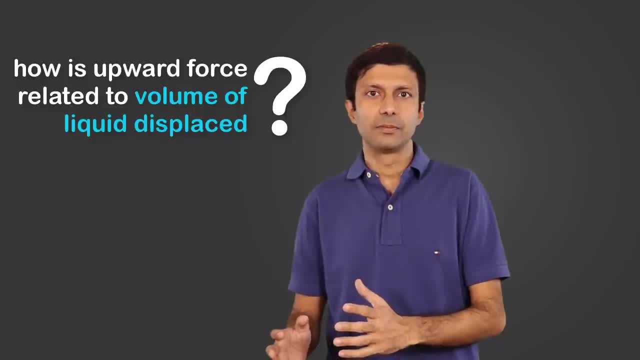 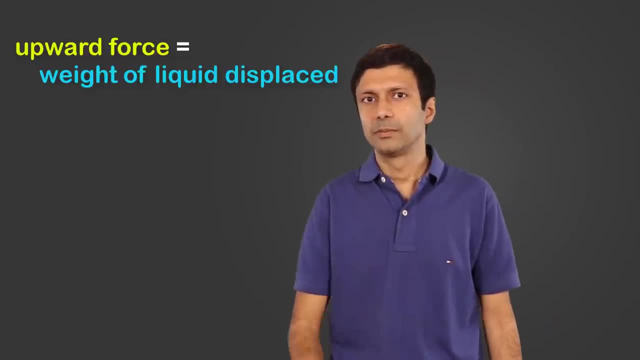 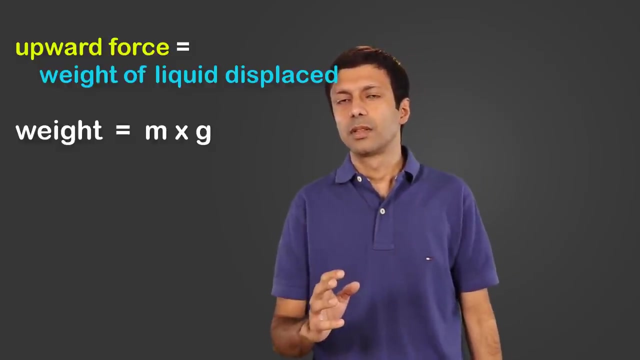 It is related to the volume of the liquid displaced. We have learnt that the upward force is equal to the weight of the liquid displaced And we know that weight is mass of the liquid into g, where g is the acceleration due to gravity. Now, what is the formula of? 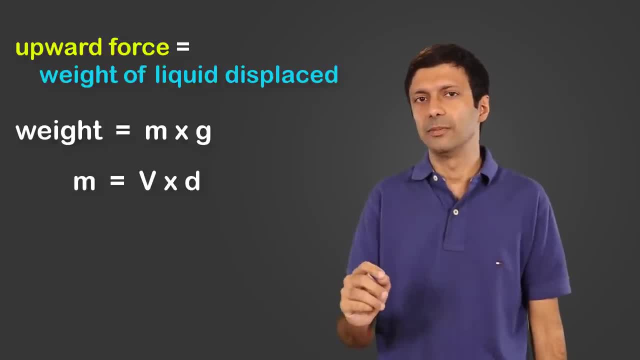 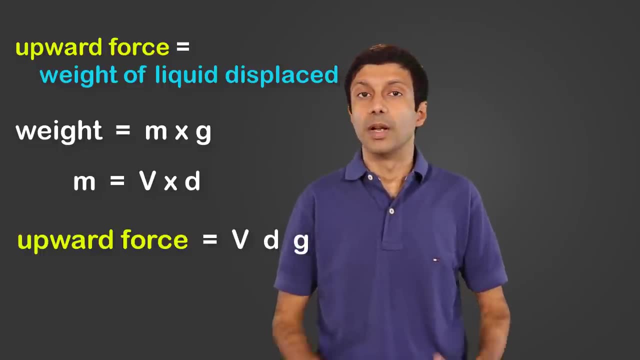 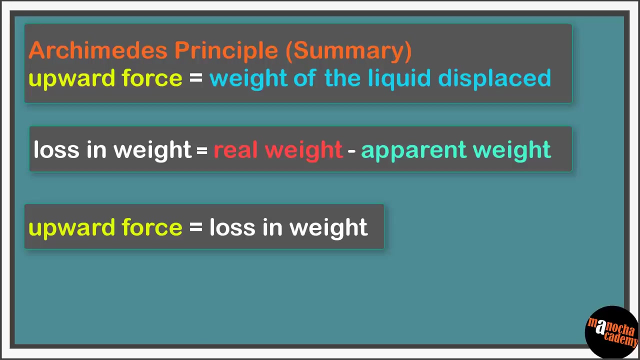 mass. It is volume into density. So we get that the upward force is weight of the liquid displaced. So let's go ahead and add this formula and the mnemonic that we learnt to our board. Here's a summary of what we've learnt in this video so far. I highly recommend you to pause.